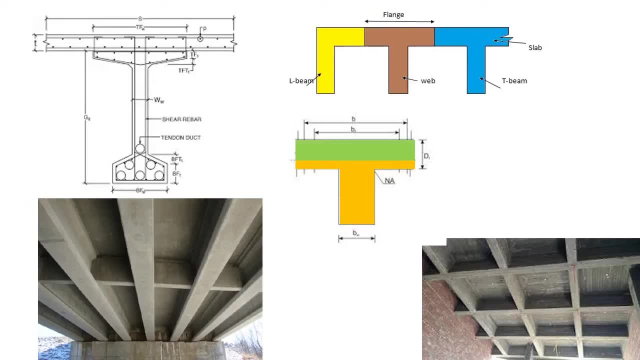 so let's start so at the very first, i would like to, uh, take example from two different structures. first, one is the bridge, one, okay, and here you can see, this is the pyre and this is the girder. this is the girder and this is the deck, okay, 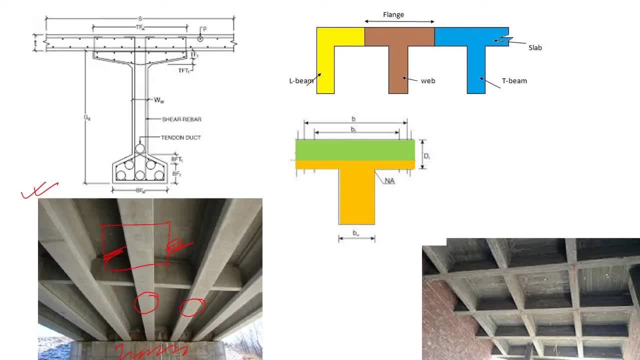 now, if i simply cut any particular section, it looks like a t beam. okay, and here you can see: this is the deck, of course, and this one is the girder, correct, and this is also applicable for this roof slab, where this is the slab and this are the beam. okay, again, if you cut any particular. 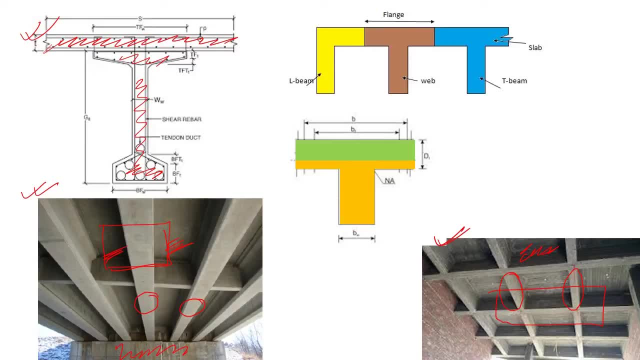 section, you can say that it looks like this one: okay, and here you can see that any particular middle beam is look like a t beam okay, and in any type of tv, whether it is in case of bridge or in case of a, simply our roof slab, the top most part. 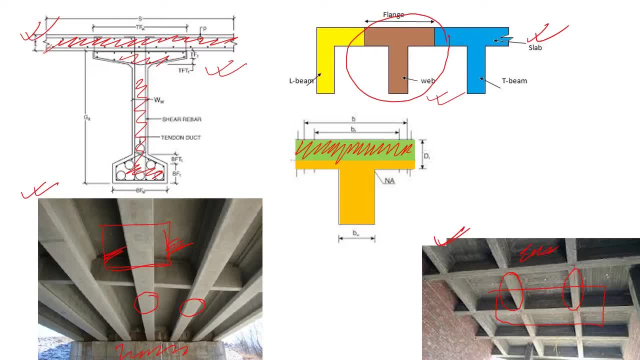 or this green part is under compression, agree, and this yellow part or the bottom part is under tension, okay. so now you have got an idea about the force coming at different part of this component, okay, so in any t beam, this top most part is in compression and bottom most part is in tension. 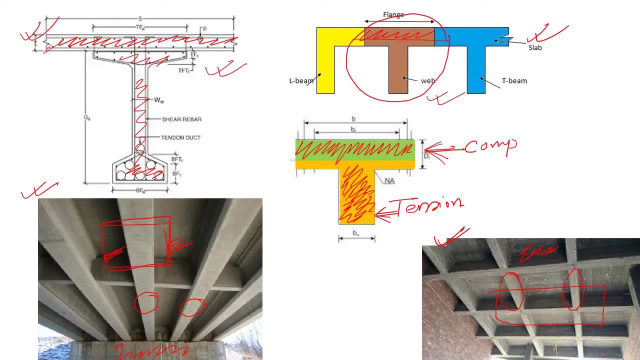 so what is the big deal? why does it matter? we need the composite construction. okay, so in case of this concrete construction, what are the backlogs? simply, they are not that much durable compared to composite construction and also in this type of uh single material construction, the material utilization is not hundred percent. 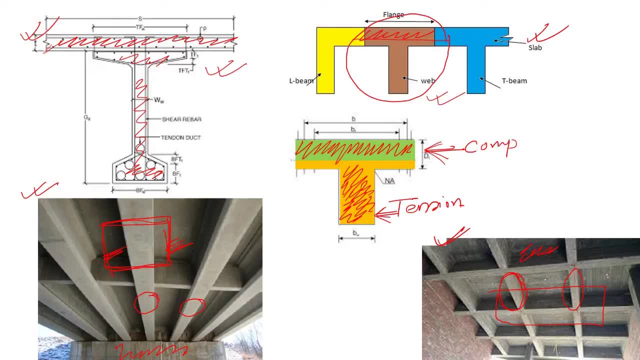 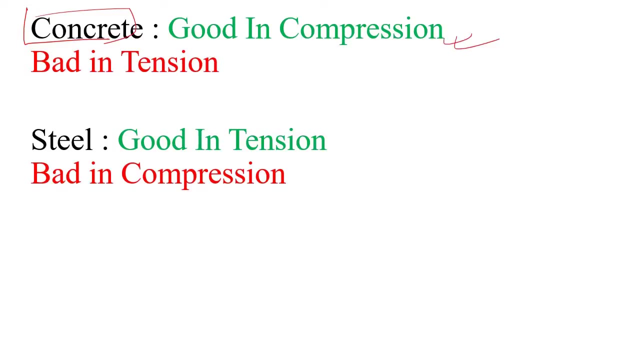 not only that, the pace of construction or the time required for this type of construction is also a large compared to the composite construction. now why? okay, you know that concrete is very much good in compression, agree, but it is very much poor under tension. contrary, still is good intention. 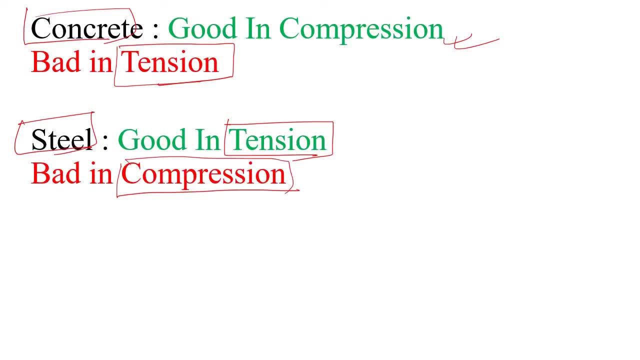 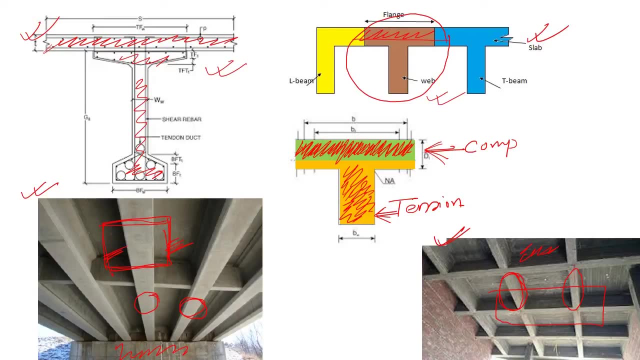 but it is poor under compression, okay. so what if? if we replace all these compressed material by concrete only? okay, we will use only concrete for compression, because concrete is good under compression, but in case of any tensioned material we will use only steel, okay, so here we will replace all this roof beam or this girder concrete girder, this girder- okay, by still. 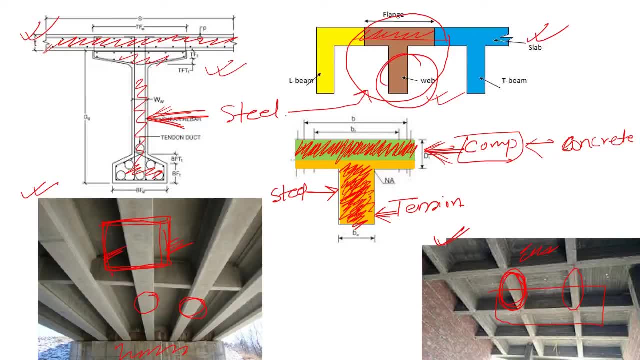 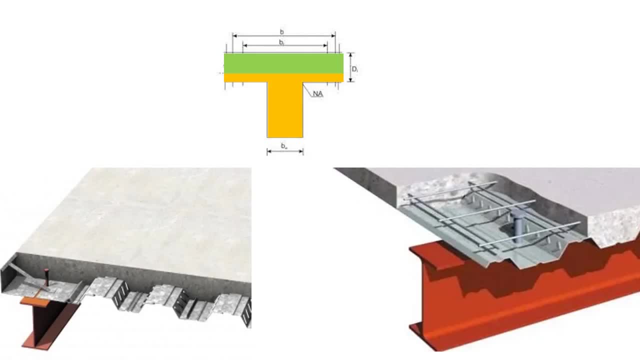 and also this one by steel. okay, so now it has become a composite girder where we are using all this compressed material as concrete and all this tension material. i am not using higherahlen layer, but it is not easy to work out what type of construction we are. 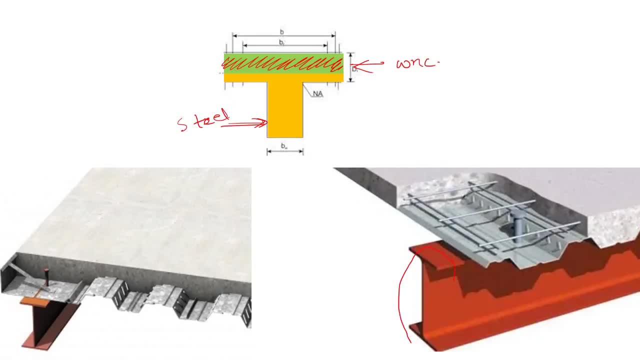 flourishing. so here it is okay. threatening material for central construction: okay, so fine, is there 1 inch longer than the range up from catch and shelter component to miss? and perfect, fine, is there 1 and 1, 1 and 1, 1, 2, 3. 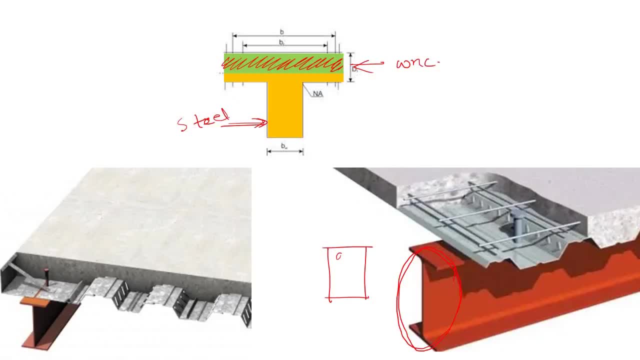 and these types of geometric visualizations we have with thisones, you might ask, okay, how the huge thickness for the base is going to be compared to the formation and temperature that is coming through by natural conditions or by raw equipment that is going to be Pike uk. 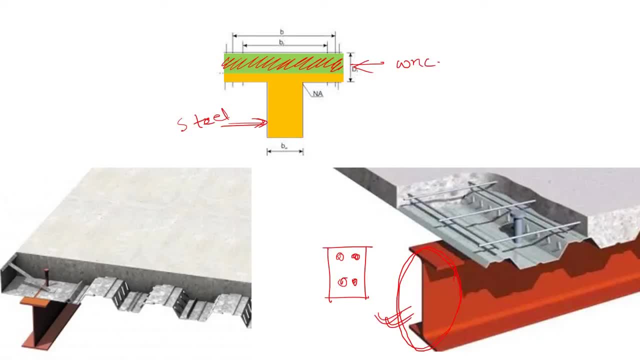 mining, you have to audit security. okay, no, yo. as for these types of structure that is going to be accepted because they not the well it has not been that. as this is made of steel and this whole zone is under tension, you can utilize this material more economically correct. and as the deck is under compression, let's use concrete. 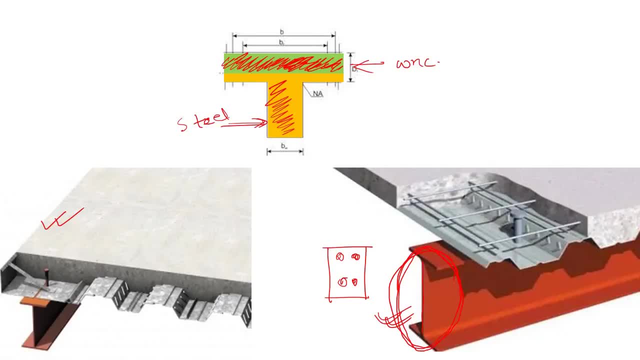 okay, so this is the concept or the fundamentals behind the composite construction. now, here you can see this particular start and also here you can see this start, why these starts are used. okay, you have understood about the use of concrete and this top zone. you have understood about the use. 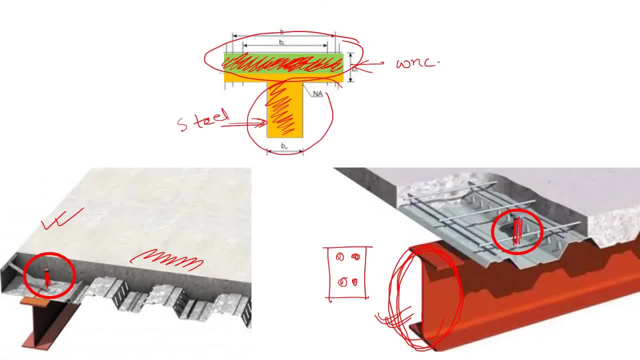 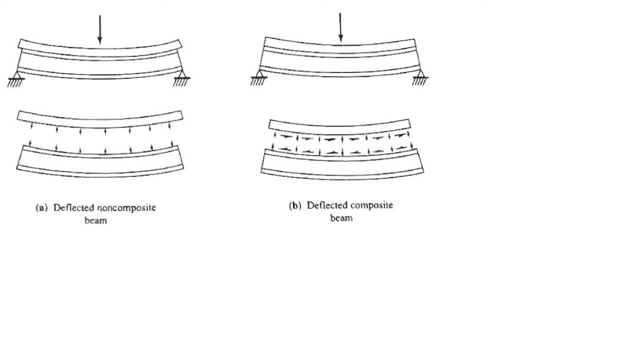 of steel under this bottom zone. now why do we need to use this type of start? okay, let's try to understand. when you are using this as concrete and this is at steel, okay, it's okay. but once you have applied your load, what will happen? they will deform separately. 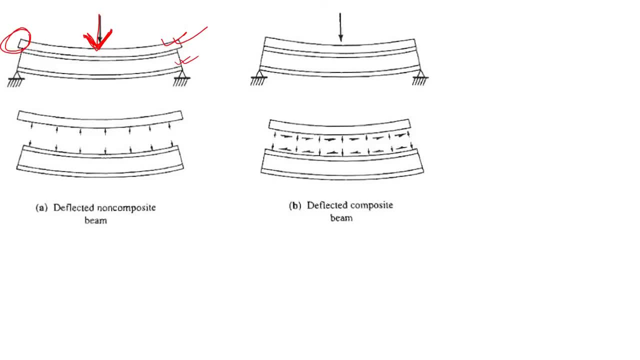 as a result. here you can see there is a slippage, okay, and also in this end you can see the slippage. that means they are not acting monolithically. so what you have to do, you have to simply connect them by some shear keys or shear stud, whatever you can call it, so that there is no 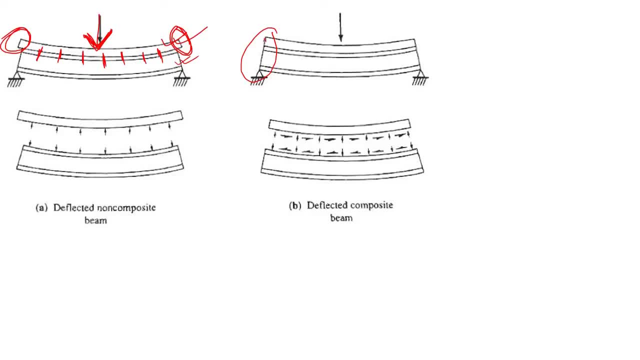 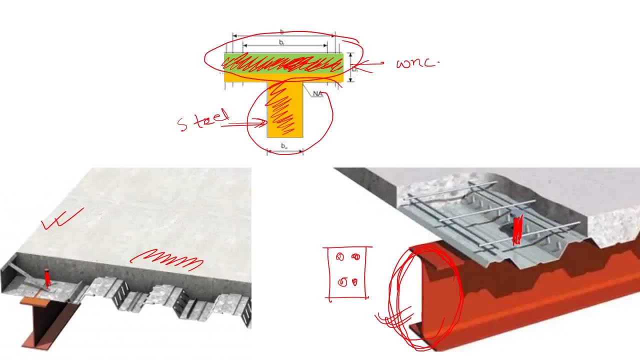 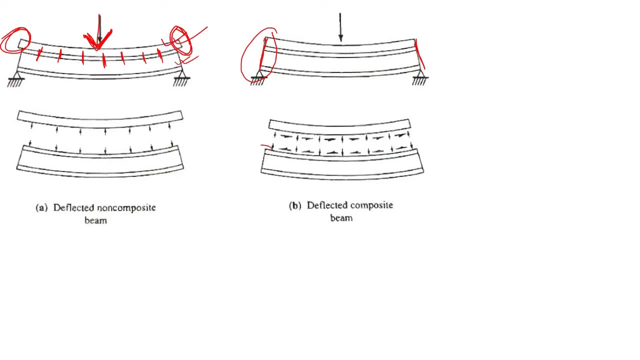 such slippage. here you can see that there is no slippage. there is no slippage. so this is the function of this shear stud, correct? this is the function of this shear stud. okay, so you have got the idea about using of steel material in tension zone, concrete material in the compression zone as well. 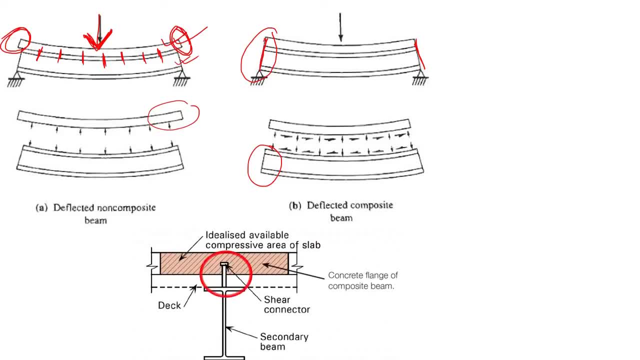 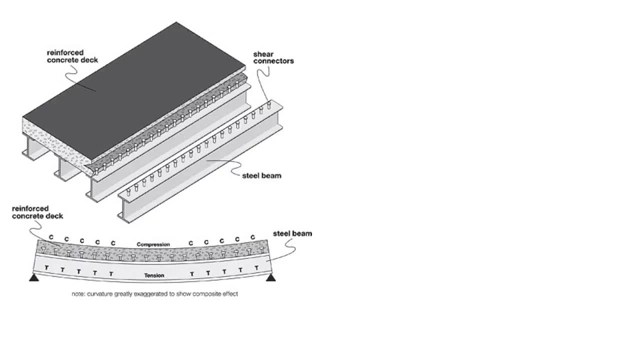 as the use of this shear stud. okay, so now let's see, after the use of composite construction method, how a bridge construction looks like. okay, so this is the joist we have used instead of concrete beam. okay, then we have placed this stud. okay, then we will place this concrete as taking material and finally it will looks like this: okay, in real cases. here is the joist. you can see, we have to press off this joist. once again, the how, but we have to press off and that will look like this: okay, then we place it back and here is this composed, this absorbing material and, lastly, it will take a position. okay, here is the how, and after this you'll have to write down these, so the joints to which is somewhere. okay, so do we have. i, we appreciate this beforehand. the bones are going to flash, cast noise, or even that preceding job. you you'll also have to paste the導 lit so that, for example, after the jump into this, Иguar's�иль. 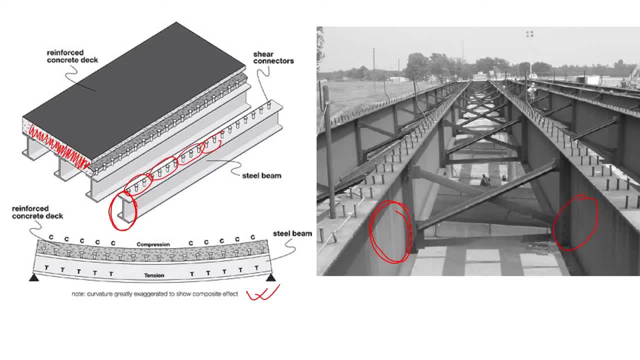 Okay, you can place these breaking with some time and then after this you'll have to Qing Luaaa. this is the joist, and we have already placed the stud to resist the slippage between steel and concrete, and after that we will place our concrete. okay, here the concrete has not been placed yet.